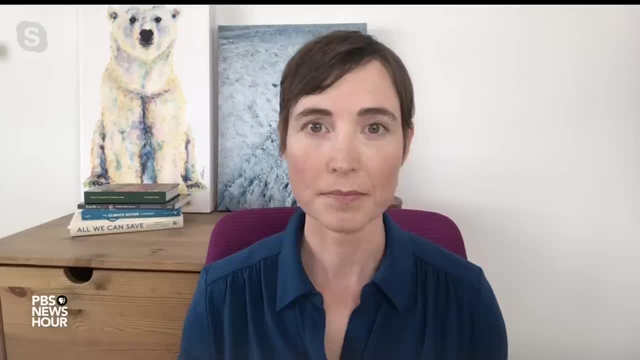 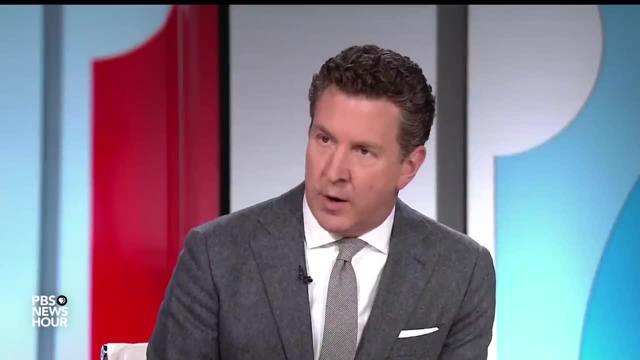 deputy lead scientist at the US National Snow and Ice Data Center. She was not involved in this most recent study. Twyla Moon, great to have you on the NewsHour. You were the researcher that I quoted there as describing this as a devastating trajectory. Can you explain why it feels that way? 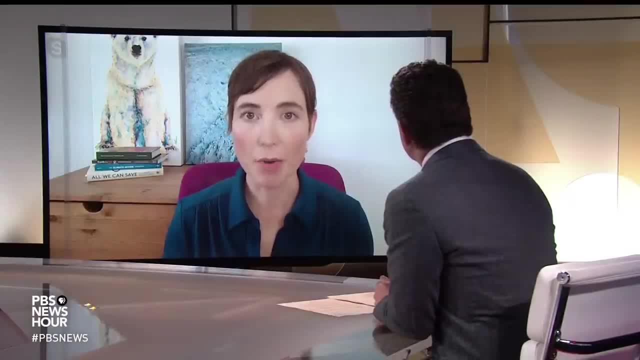 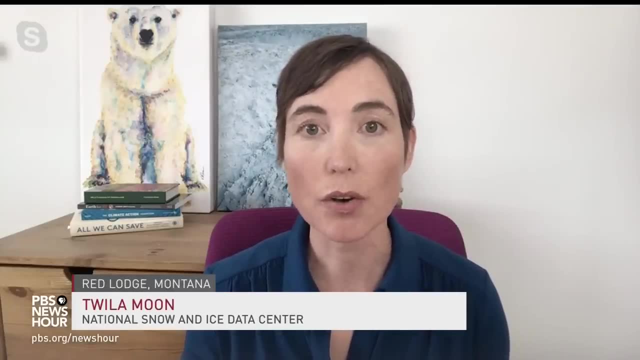 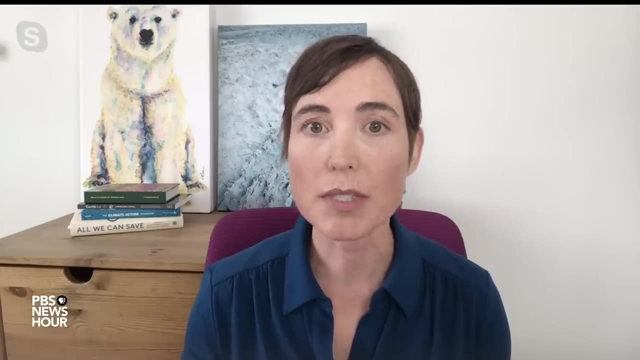 to you. This is something where, as we're losing ice around the world, the biggest impacts are felt by those people who are actually far from this ice And living in coastal regions in North America, Asia, Africa, all around the world, And so seeing this continued rise in ice loss is really not good news for dealing with sea. 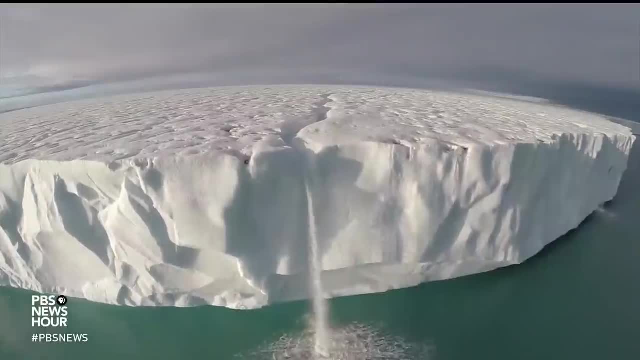 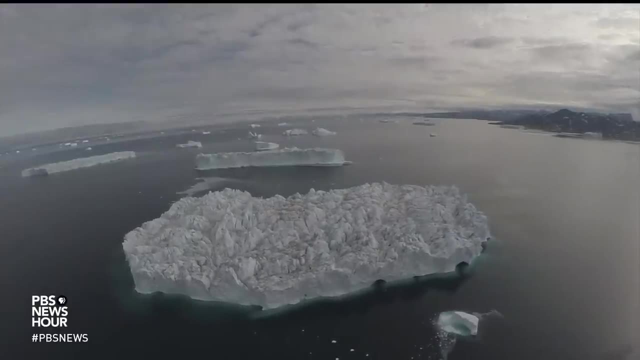 level rise, But I do want to be clear that this is not an inevitable trajectory either. WILLIAM BRANGHAM, We're talking about ice that used to live up on land, now melting, disappearing and ending up in the oceans and driving up sea levels. 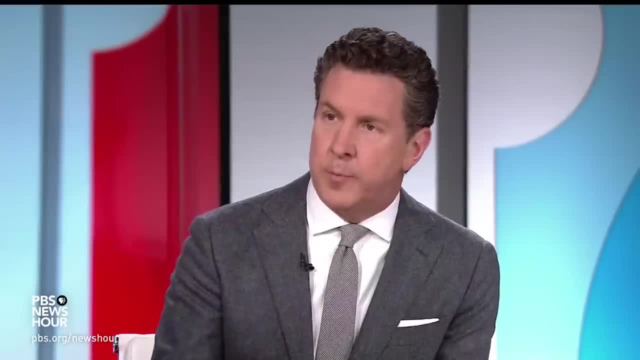 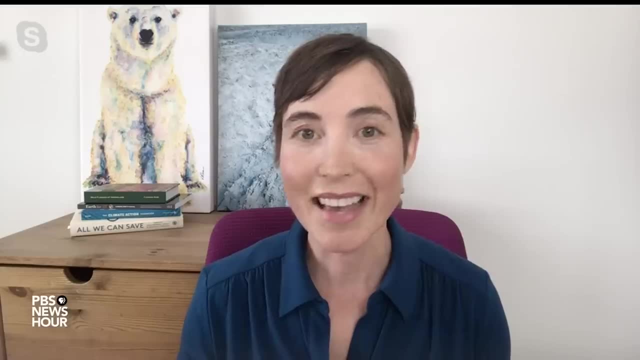 Sometimes I think the numbers here. when we talk about billions of tons, it's hard for people to fathom what we're talking about. What are the literal downstream consequences for communities all over the world? DR ANNE-MARIE BAUER. Yeah, I understand how the numbers can seem hard to deal with. 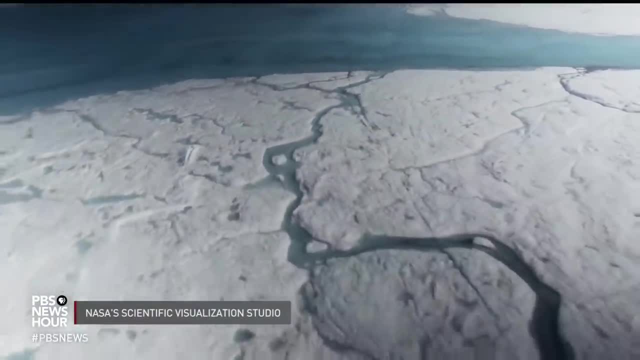 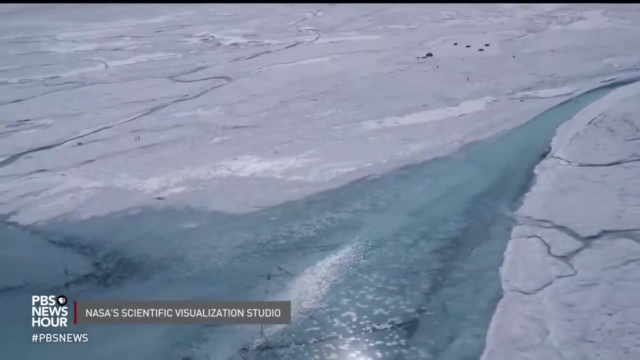 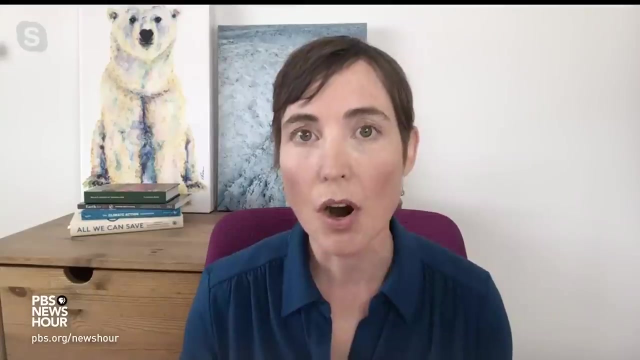 It's important to remember, the Greenland ice sheet covers the world's largest island. Antarctic ice sheet covers a continent, So these are very vast areas that are hard for us to imagine And, as we're losing ice from these areas, what we see arising at our coasts are things like coastal erosion, where we're losing land. We might have ocean water inundating our freshwater resources or causing problems with water and sewer systems. Or we might see flooding in areas that have never experienced it before, even further inland from the coast, and also areas that do experience flooding having that. 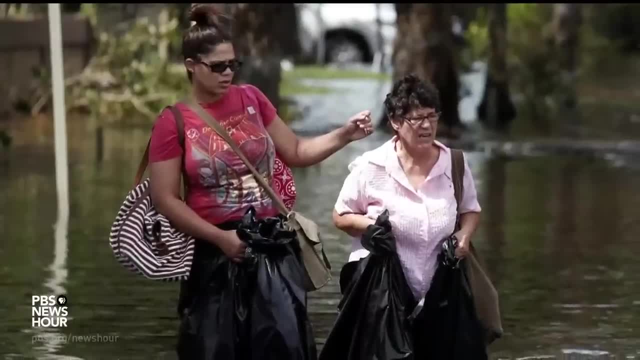 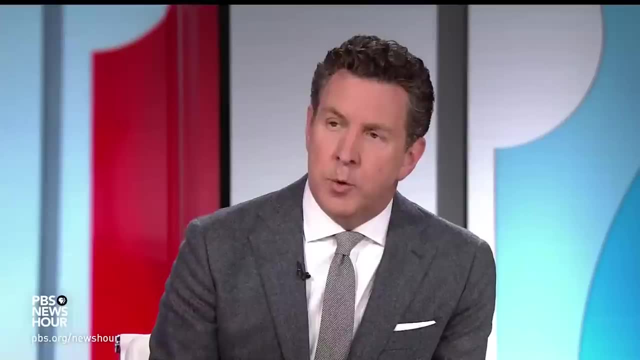 occur more and more often. So these are impacts that we feel around the world And those for those of us who have felt very far from ice. WILLIAM BRANGHAM, You were saying that this is not baked in, that we can act on this. 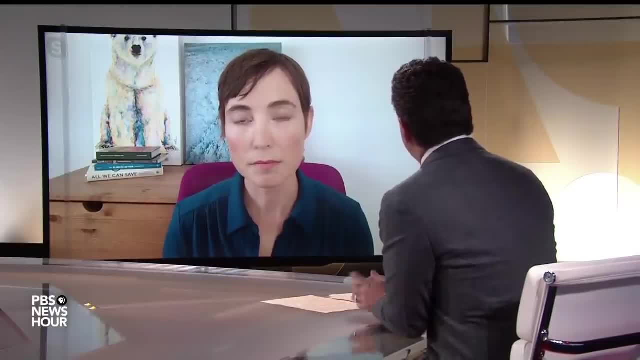 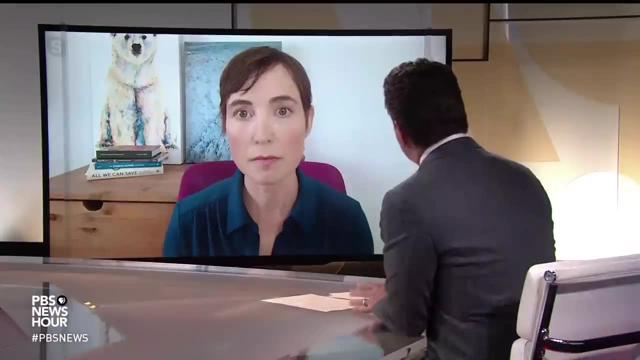 But there is an enormous amount of carbon that we have already put up in the atmosphere. I mean, even if we stopped today emitting carbon 100 percent, wouldn't there still be some of this pollution and warming? that is baked in DR ANNE-MARIE BAUER. Yes, that's correct.